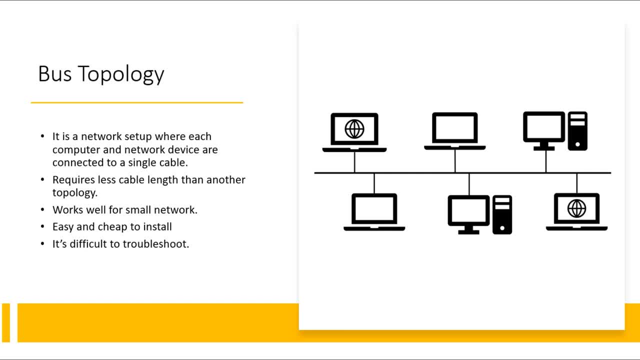 than another topology. Some of the disadvantages of using a bus topology is that it's difficult to troubleshoot. Bus topology is not great for large networks. It can be hard to troubleshoot individual device issues and it hard to change or move the devices. 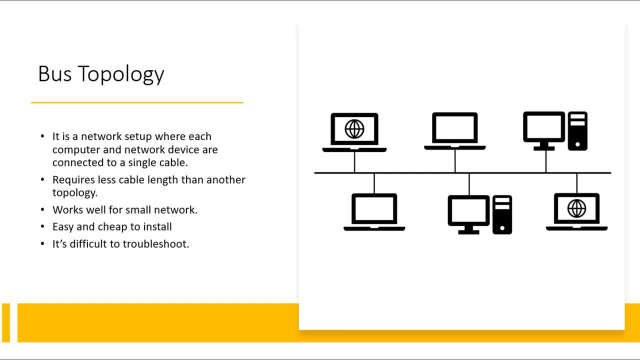 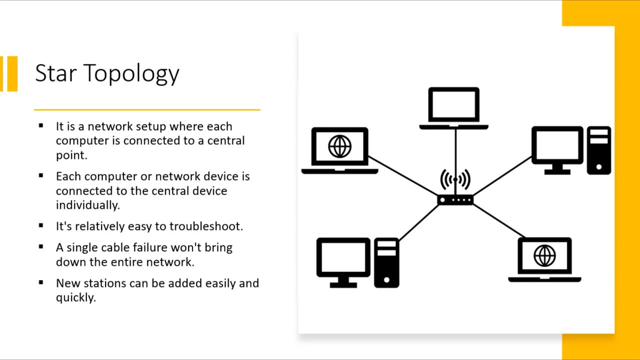 In a bus topology it can be difficult to identify the problems because every device in the network is connected to one single cable. This means that any fault in the cable would bring the whole network down. Star topology. Star topology is a network setup where each computer is connected to a central point. 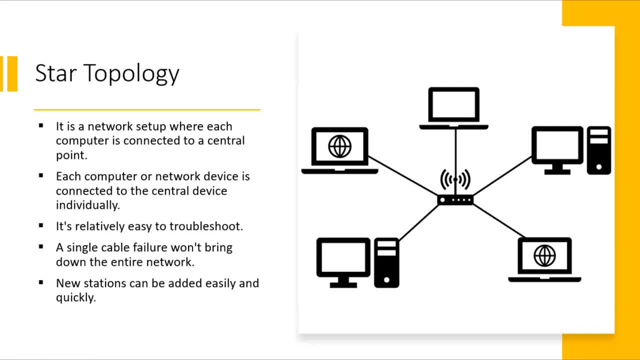 usually a switch or a hub with their own network. Musik Startupology is widely used in today's networks. It is used in most large and small networks. One of the best features of startupology is that each computer or network device is connected to. 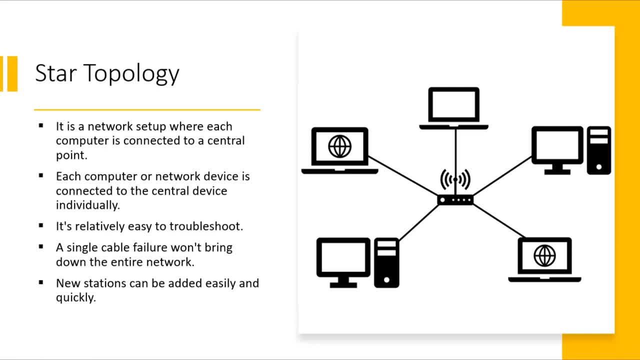 the central device individually. If one cable fails, it only brings down the machine or network segment related to that point. This makes the network much more, a lot easier to troubleshoot. 而已. One cable two times, three times, five times, That may increase some link between areas as shown, or decrease the number of devices. One cableum by aspect of one cable is in the center, on the upper left line of the network and free from some algo of. 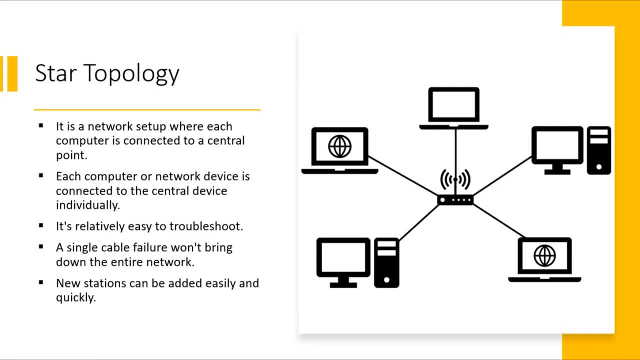 One cable failure will not bring the whole network down. Another great thing about a star topology is that it is easier to add or move the devices. All you have to do to add a new device is to run a new cable and connect it to the central. 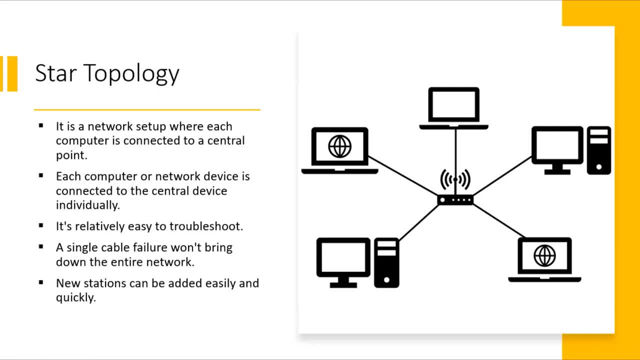 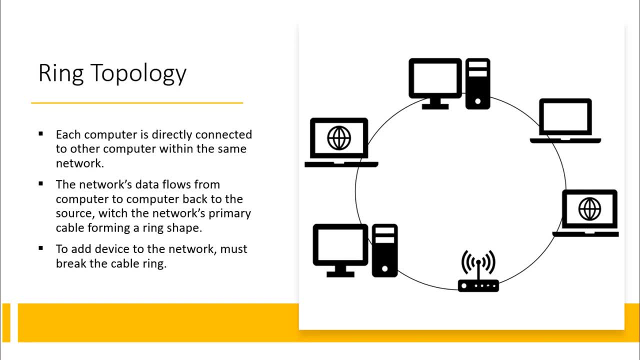 point, which is the switch or hub Ring topology. In ring topology, each computer is directly connected to other computers within the same network. The network's data flows from computer to computer back to the source, with the network's primary cable forming a ring shape. 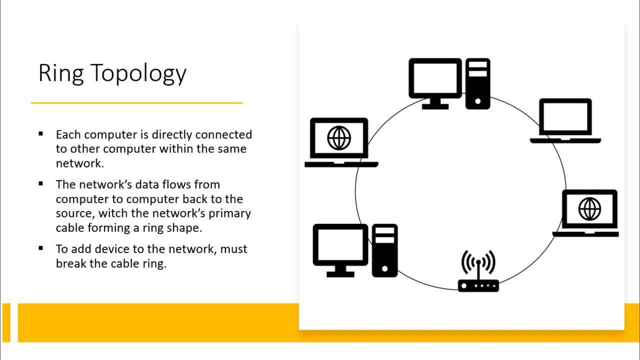 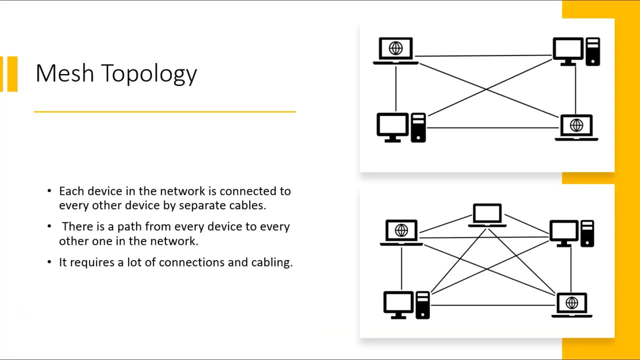 This topology has a lot in common with the bus topology. If we want to add a device to the network, we must break the cable ring, which is likely bringing down the entire network. This the reason why ring topology is not very popular in today's network. 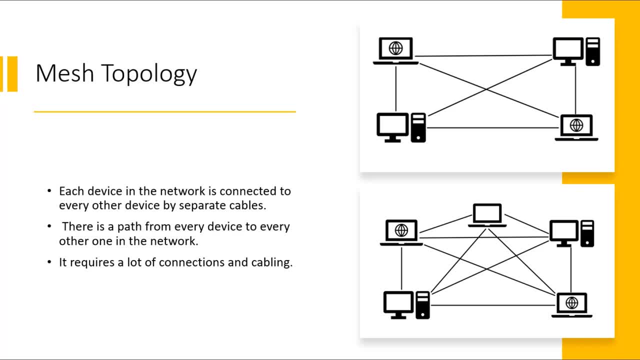 Mesh topology Each device in the network is connected to every other device By separate cables. In a mesh topology, there's a path from every machine to every other one in the network. This topology is very expensive to install, since it requires a lot of connections and